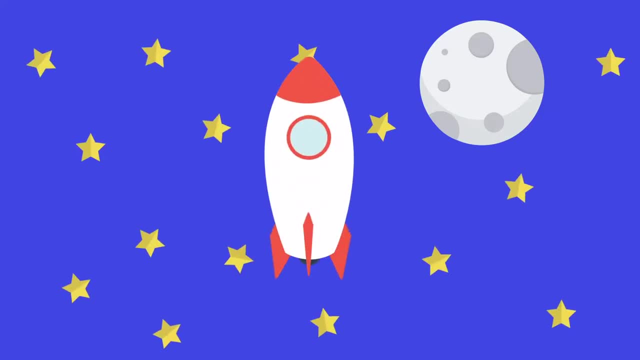 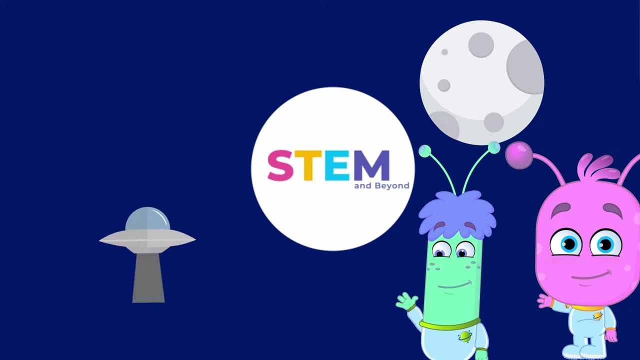 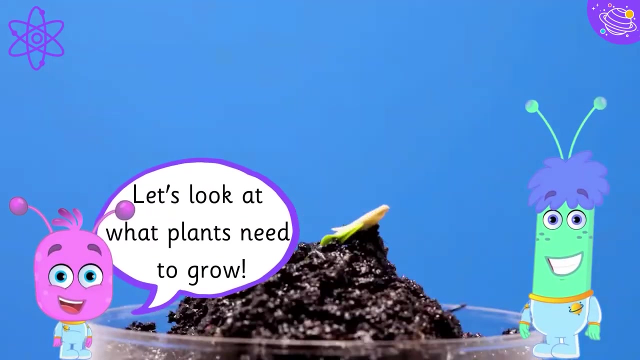 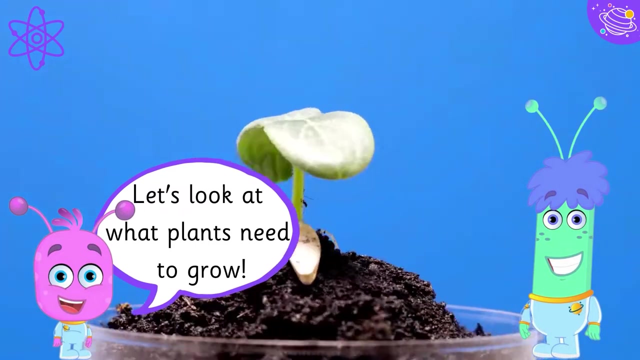 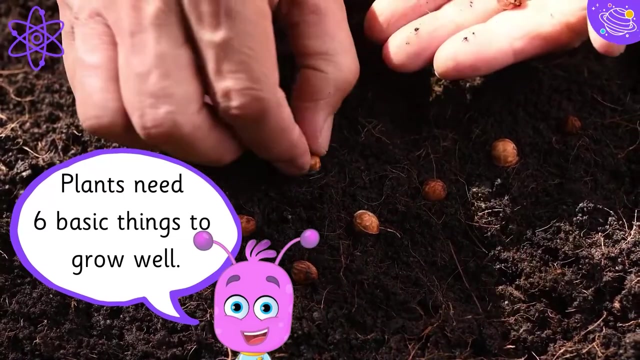 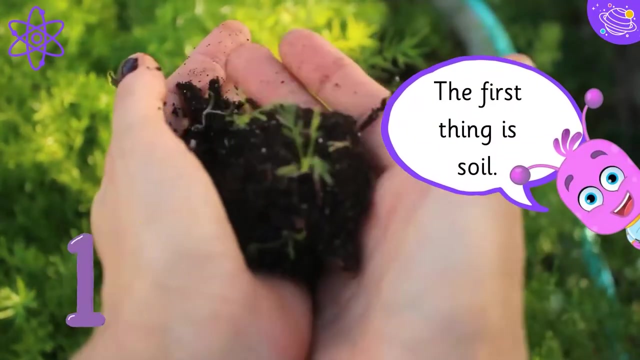 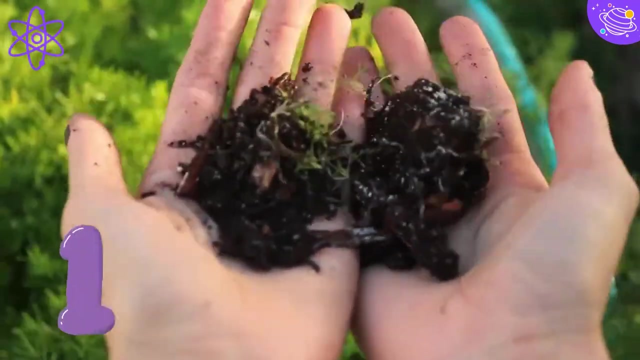 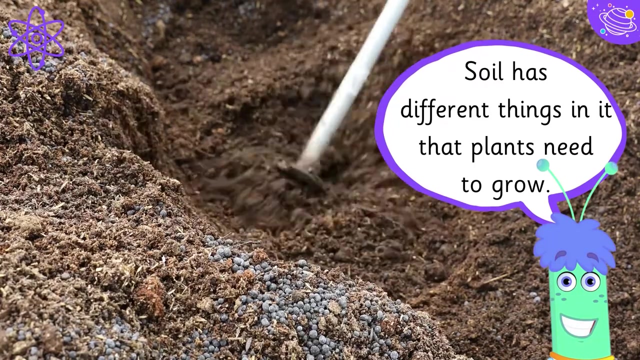 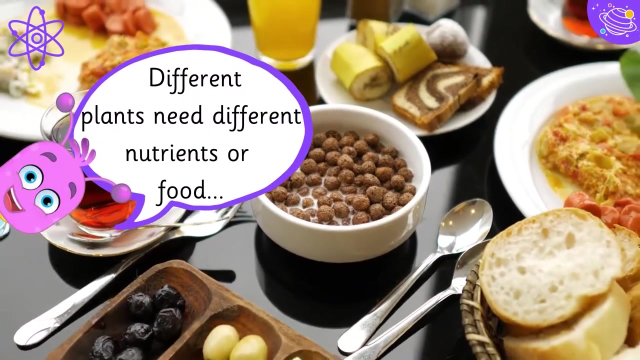 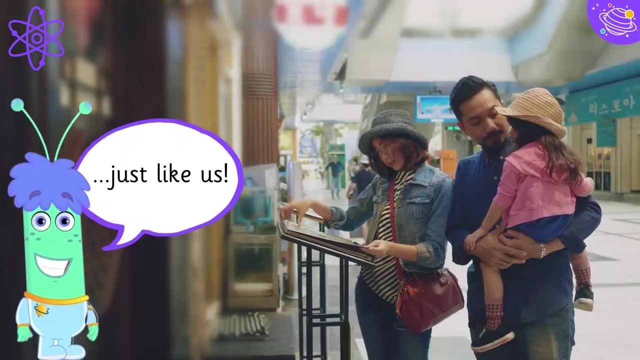 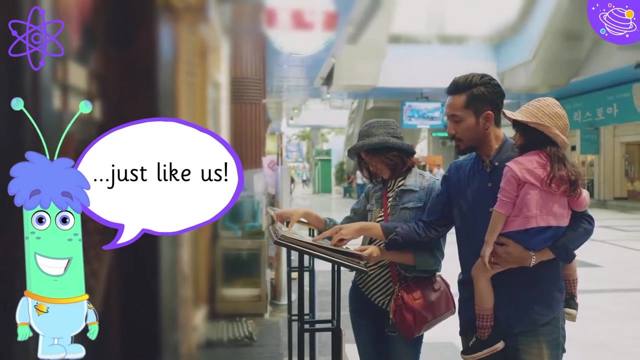 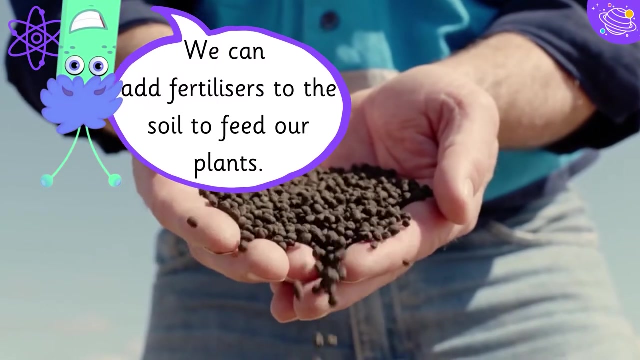 Let's look at what plants need to grow. Plants need six basic things to grow well, The first thing is soil. Soil has different things in it that plants need to grow. Different plants need different nutrients or food, Just like us. We can add fertilisers to the soil to feed our plants. 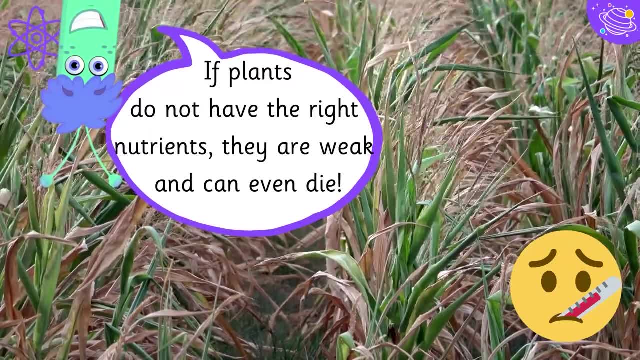 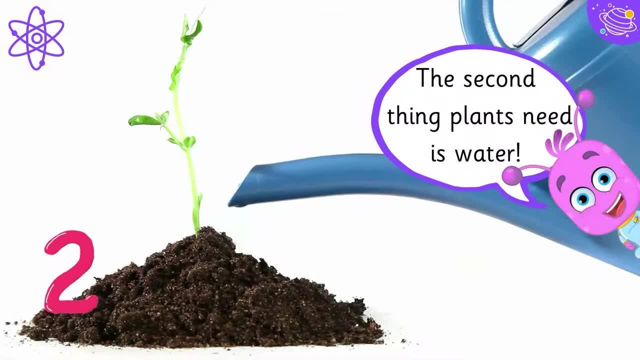 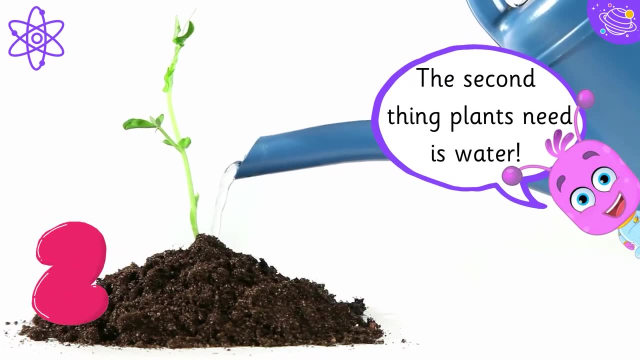 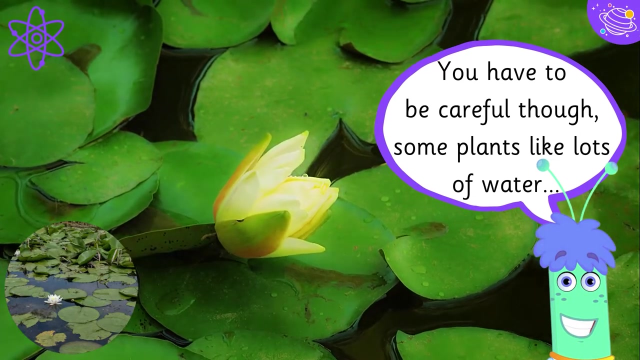 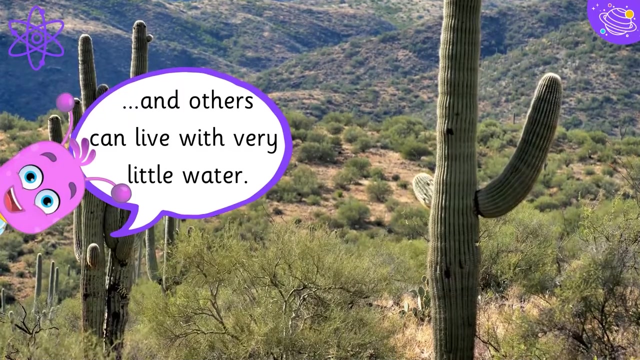 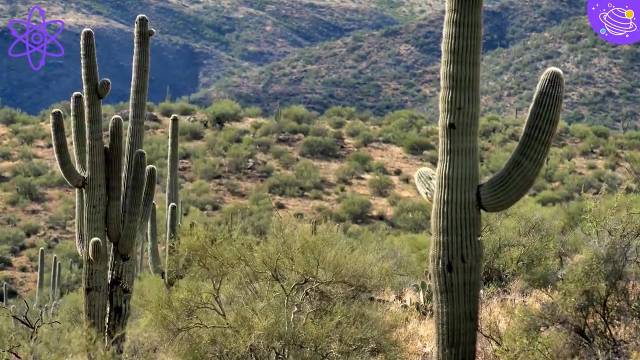 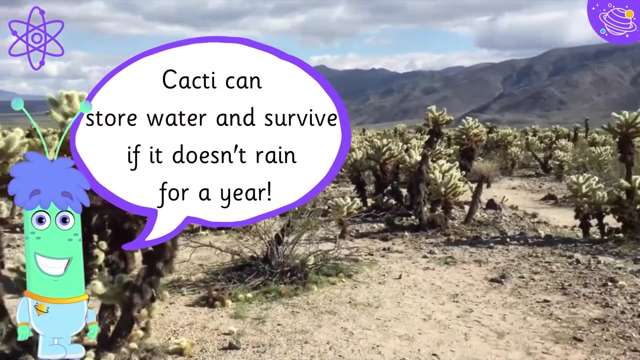 If plants do not have the right nutrients, they are weak and can even die. The second thing plants need is water. You have to be careful, though. Some plants like lots of water And others can live with very little water. Cacti can store water and survive if it doesn't rain for a year. 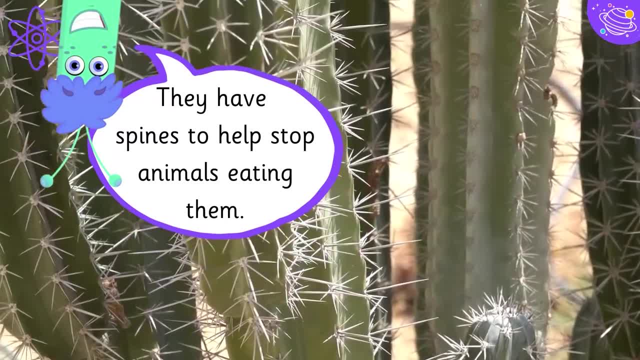 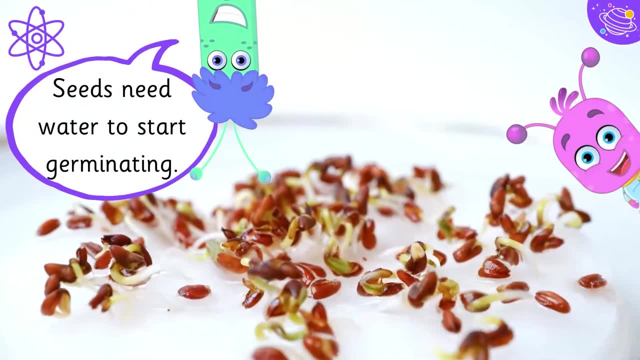 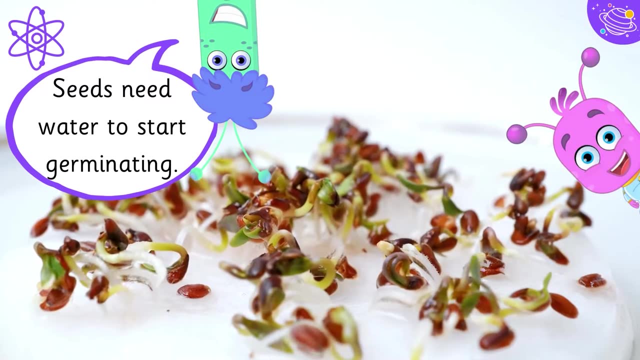 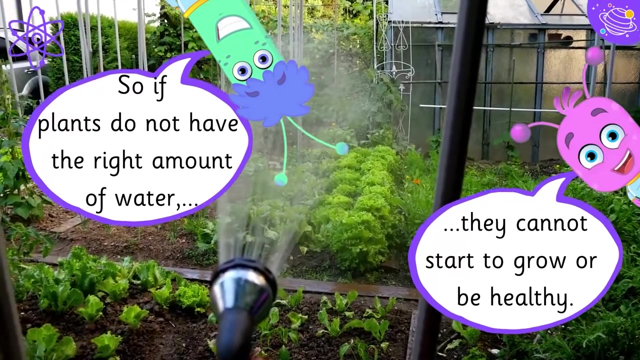 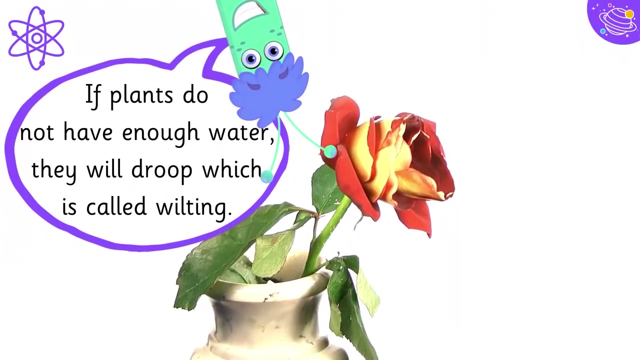 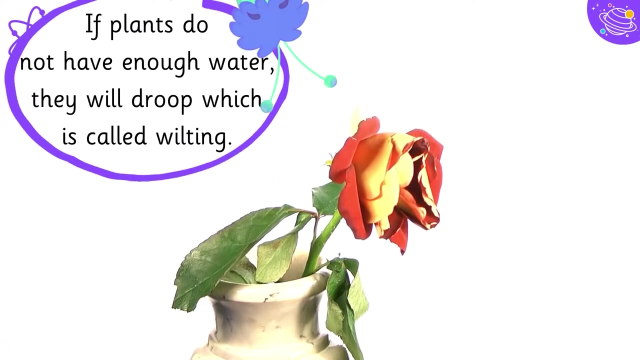 They have spines to help stop animals eating them. Seeds need water to start germinating, So if plants do not have the right amount of water, they cannot start to grow or be healthy. If plants do not have enough water, they will droop, which is called wilting.